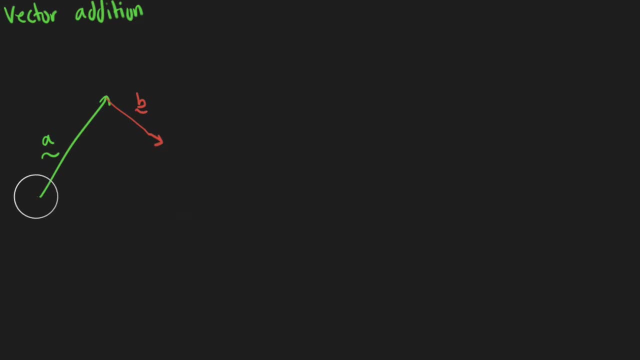 then it's really easy to add them. You just start from the tail of the first one and go to the head of the last one, right? So this is A plus B. Okay, so I said head to tail. What if I had taken this up and attached this head to this tail instead? 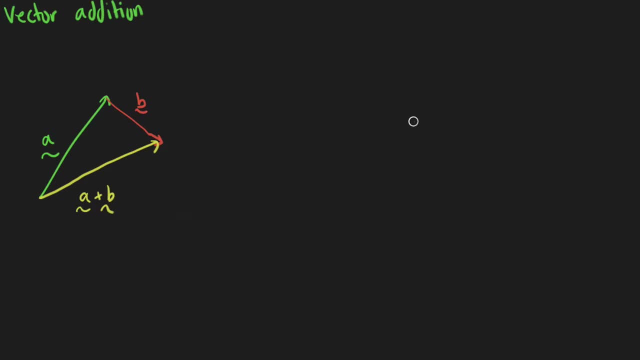 Well, it turns out you would get the same vector, So it doesn't matter, You would get the same answer. All right, so I'll try to draw them the same. So that's A, And let's say this is B, right? 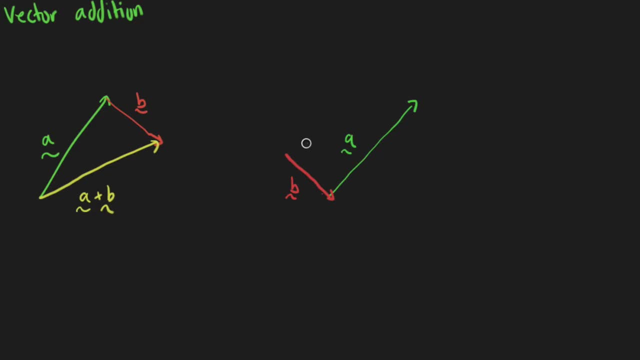 So then, A plus B, or here we're doing B plus A, which is the same as A plus B, would be there, right? So A plus B, And you can see from comparing this and that that they have the same direction and the same magnitude, right? 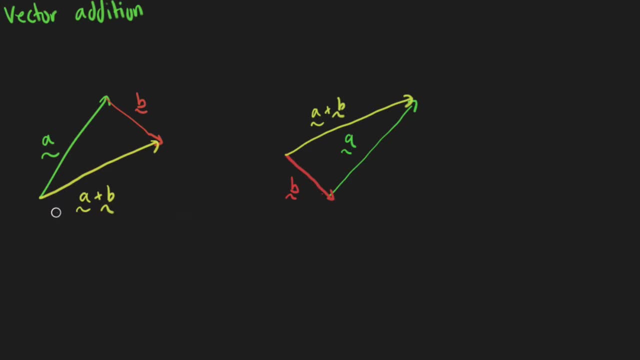 Obviously, my diagram is a bit rough, but if you were to use a ruler and perhaps measure the angles, that would be the same. So this is the geometric way, or the graphical way, of representing vector. addition And subtraction is the same thing, except, you know, you can think of subtraction as just. 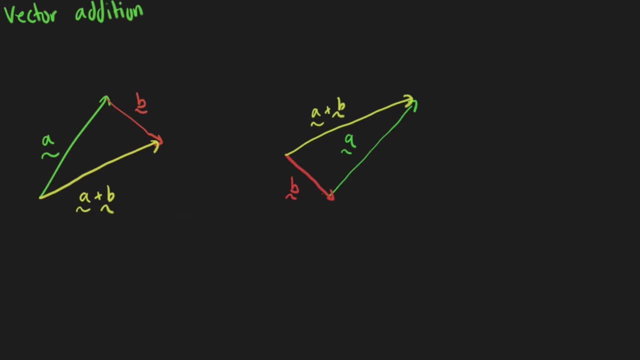 So, if you had to, This is A plus B. If you had to do A minus B, the B would just be. This would be facing the other direction. right, That's minus B. That's because the minus out here just changes the direction. 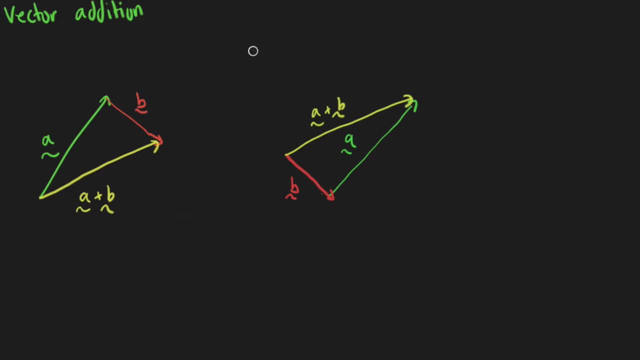 Anyway, let Let's look at the algebraic representation of addition. So what I will do is I'll rub this one out just to make some space. Okay, let's say that A is equal to 4i plus 7j, right? 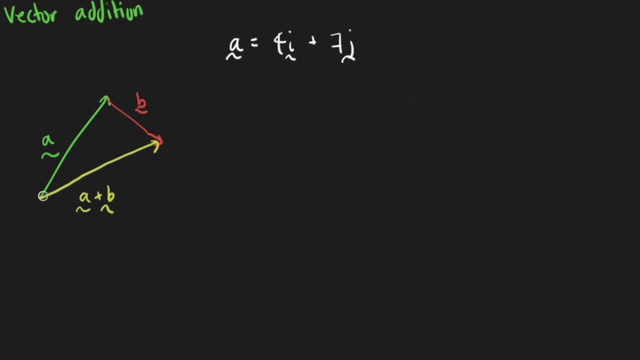 So it goes 4 right And then 7 up. This one B could be Perhaps 6i and 5j right. And adding vectors is very simple. All you do is add the individual i components and the j components. 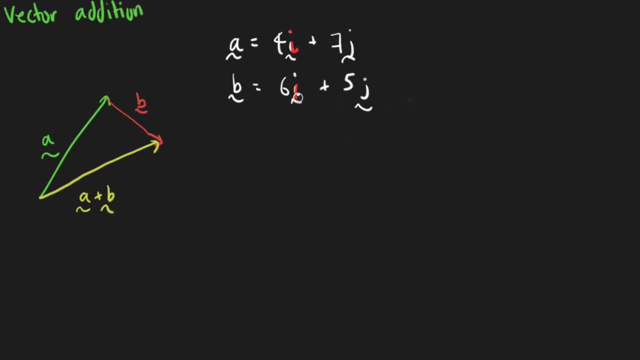 So we're going to add the i's together right, And the j's together right. So I'm going to. You can really just do this in one step, But just to illustrate it and to make sure you guys aren't missing anything. 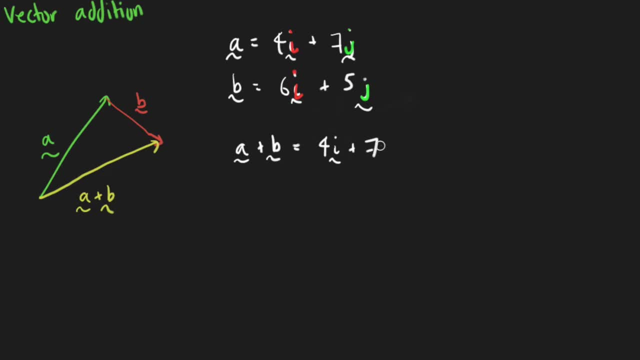 I'm just going to write it all out. So A plus B is 4i plus 7j plus 6i plus 5j. So I've just written in the values of A and B. Next thing you would do is collect the like terms. 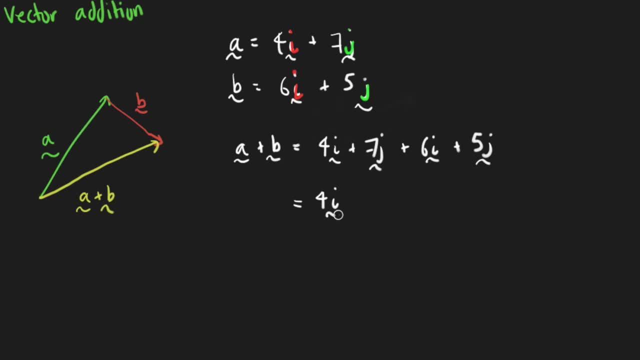 So you've got the. So bring the i's together and the j's together, So this becomes 4i plus 6i plus 7j plus 5j, And then it's really simple: You just add the i components together. 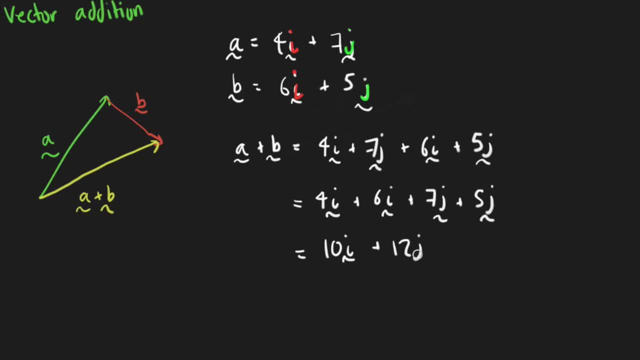 That becomes 10i plus 12j. So you add the i components and the j components separately And that's it, And maybe you could call this another vector. You could maybe call this C. Yeah, but you don't have to do that. 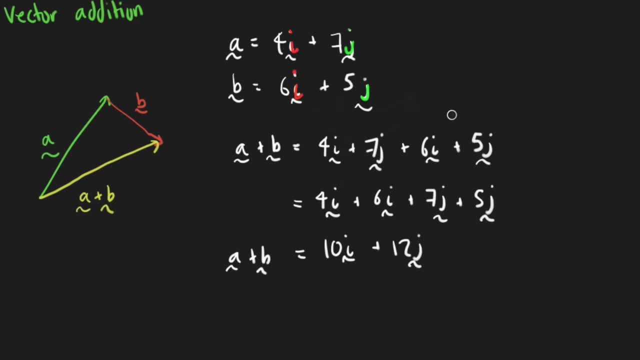 So the algebraic sort of representation of this is just that. And just remember that you can, Like I said before, this can be in another notation, which is 4, 7.. This could be 6, 5. In that case, if you were adding them together, it would just be 4, 7 plus 6, 5,. 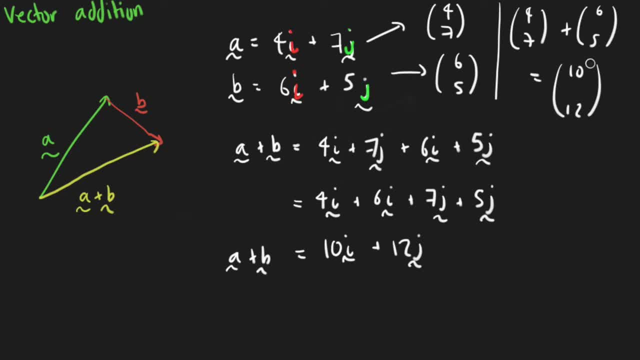 which gives you 10,, 12,, right, And that's the i component, That's the j component, just like you have here. Okay, let's do. There's one more thing I wanted to get through, which is scalar multiplication. 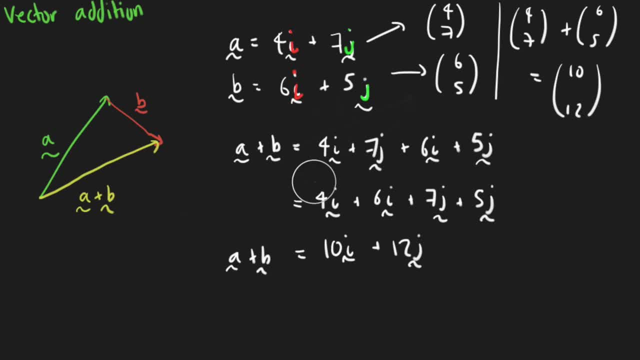 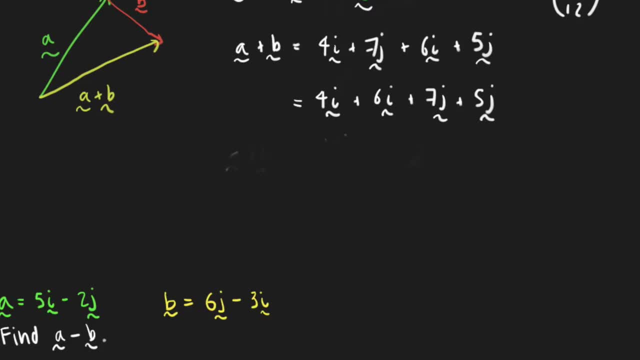 I'm just going to go through that really quickly because that will not take long. Actually, what will take long is me rubbing all that out. So these are some questions that I had, but I will go through them in a different video, just so the video doesn't go too long. 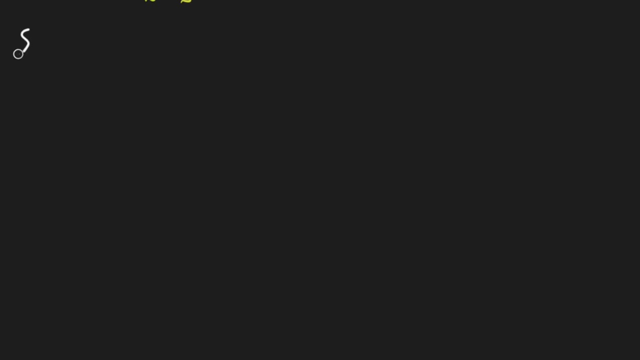 Okay, so scalar multiplication- All right. so what that means is you're multiplying a vector by a scalar, And that's really simple, because it will only take a minute to explain. So you have a vector. Let's say that's a right. 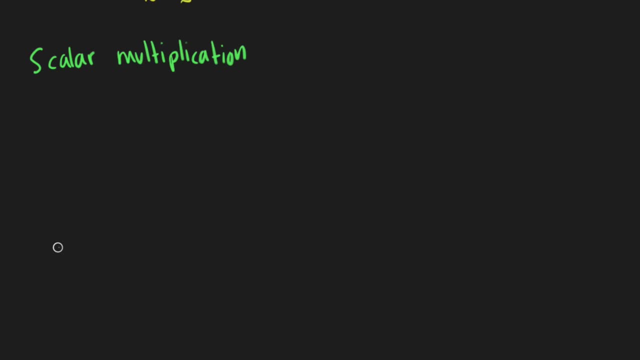 And what if? Actually, I'll make it a little bit smaller so that everything fits. Let's say you wanted to find 2a. What's 2a? 2a is just a multiplied by 2.. Now, 2 is a scalar right. 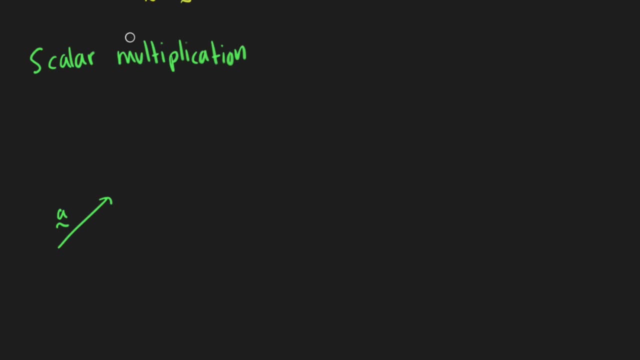 Because it's just a number 2. It doesn't have any direction associated with it. That's why it's called scalar multiplication. So 2a would just be There. 2a: You literally just multiply the length by 2..